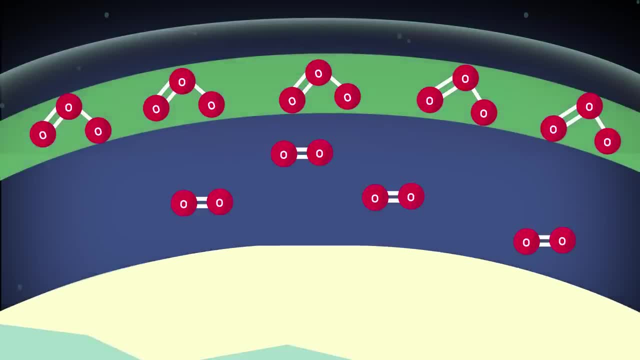 With the oxygen in place, ozone could form in the upper atmosphere, so preventing dangerous ultraviolet light from the sun reaching the land. This was a sign that life had taken hold. With the oxygen in place, ozone could form in the upper atmosphere, so preventing dangerous ultraviolet light from the sun reaching the land. 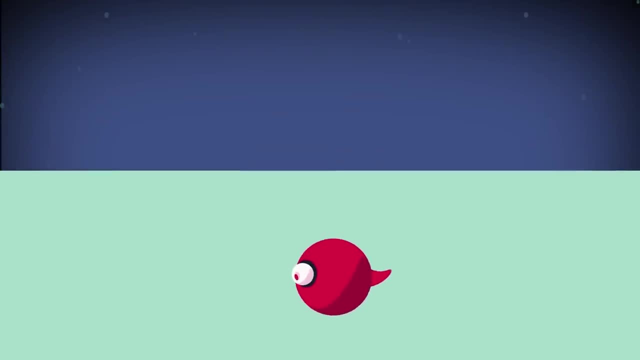 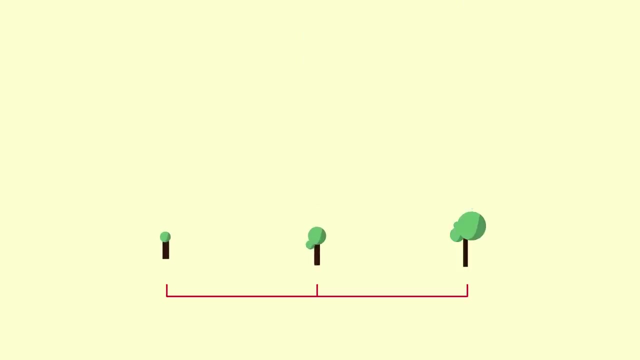 Before then, life could only exist under the water, where the UV could not reach. However, life did not invade the land immediately the ozone was in place. It was a big evolutionary step for plants, which needed water to give them support. About 400 million years ago- 100 million. 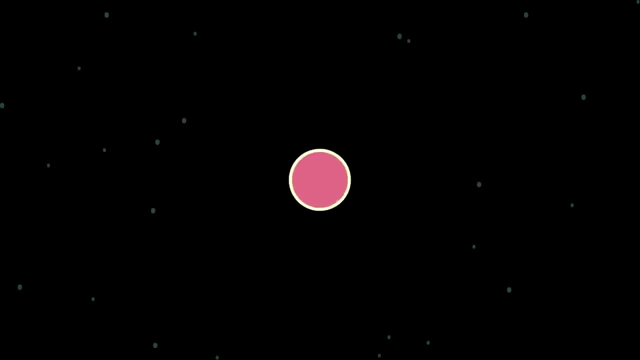 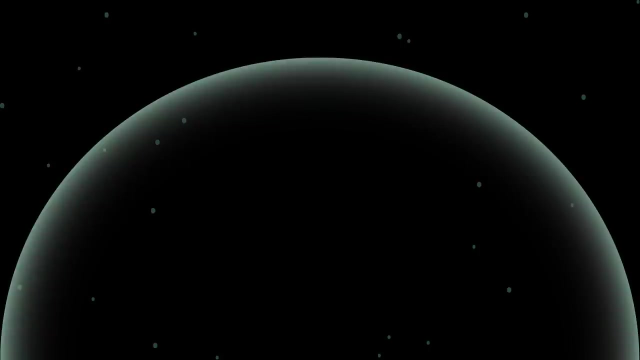 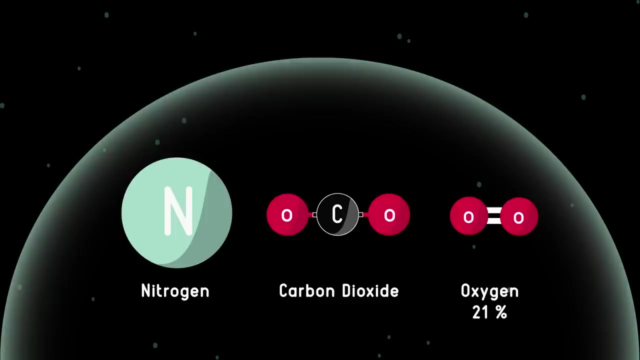 years after the so-called Cambrian explosion, life finally learnt to live on land. The atmosphere remained much the same until the last century: mostly nitrogen, with 21% oxygen and just a tiny amount of CO2, but enough to give plants their carbon during photosynthesis. 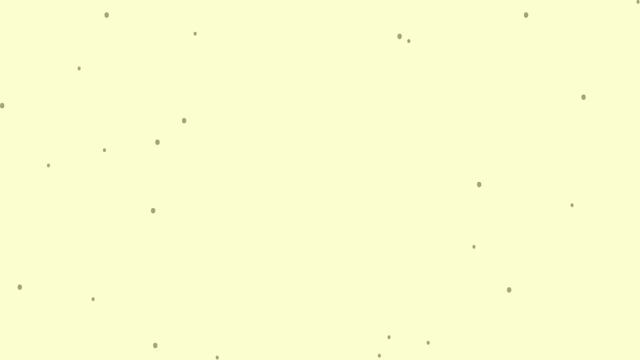 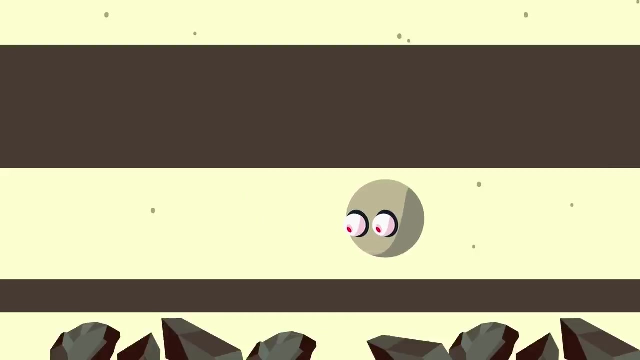 However, a hundred years ago or so, another living organism started to change the atmosphere. This organism found seams of coal and pockets of oil and natural gas underground and began extracting them and releasing them to trade, But they were in vain. They found they could notEM back in annoess. 아주 sy nem400 eandern Lavlaolved andersnya. Barbara Binar i 103' Atmosfair аnd Up physics Land. 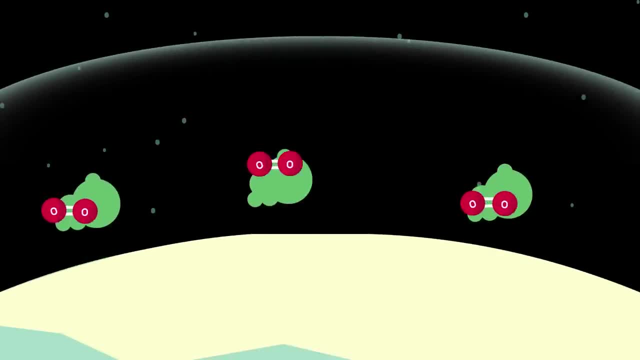 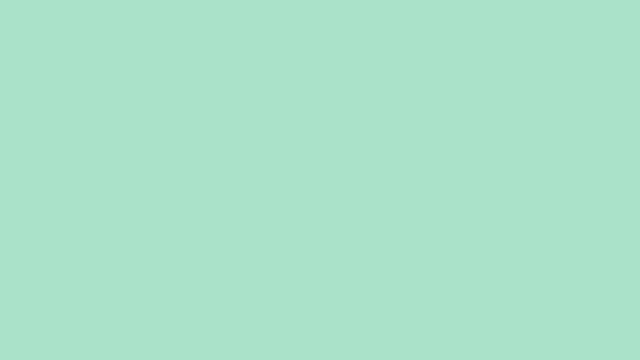 reacting them with oxygen in the atmosphere, increasing the carbon dioxide concentration. Mankind- for that was the name of the organism- also began to throw away other unwanted material into the atmosphere, and you can learn all about these in our related videos For carbon dioxide. 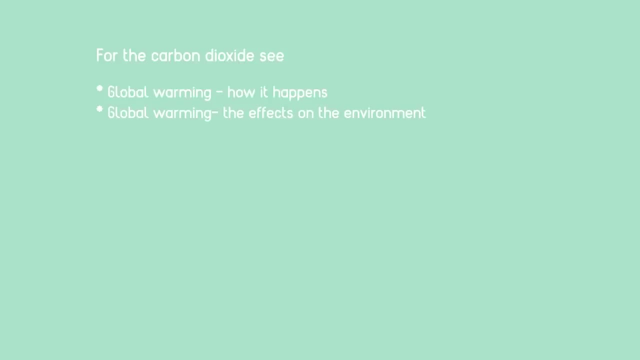 see global warming- how it happens, and global warming the effects on the environment For the acidic oxides we throw away up our chimneys and in our vehicle exhausts. see acid rain and reducing acid rain or its effects For the CFCs which propelled our aerosols but destroyed the ozone. 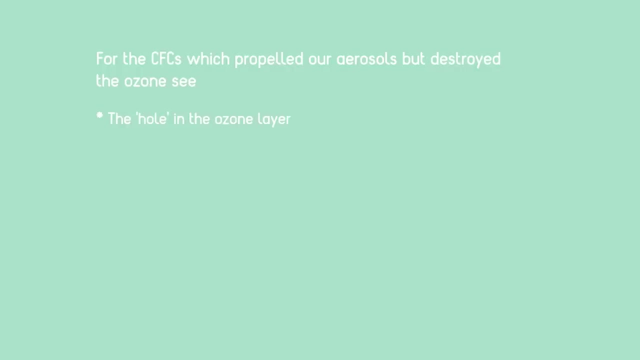 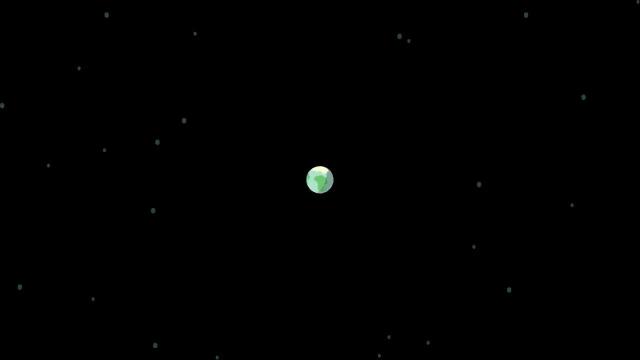 layer- see the hole in the ozone layer. And for the soot and other particles we throw away into the atmosphere, see the effect on health of air pollutants and reducing particulate soot. To summarize, it's the presence of life on this planet that has caused the atmosphere to change.